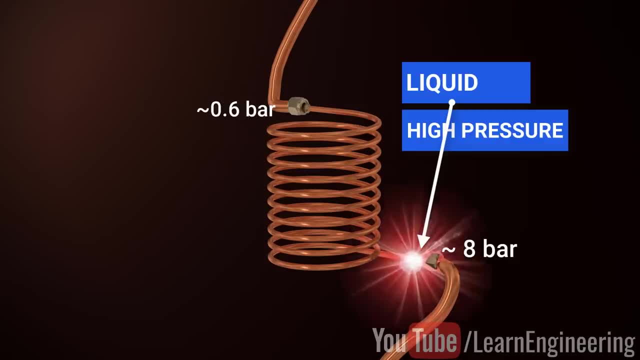 the flow of liquid that is produced by the throttling of the refrigerant. The throttling is a constant flow of liquid that is produced by the throttling of the refrigerant. The throttling is a constant flow, so a huge pressure drop occurs when the liquid flows through it. 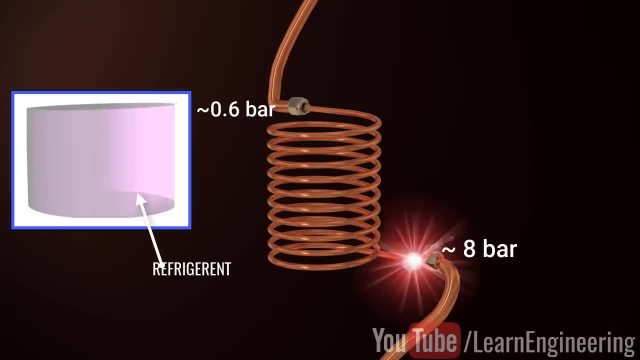 As the pressure drops, the boiling point of the liquid comes down. Thus the refrigerant liquid evaporates. The energy required for such evaporation comes from the refrigerant, so its temperature drops If you check the temperature across the throttling device. 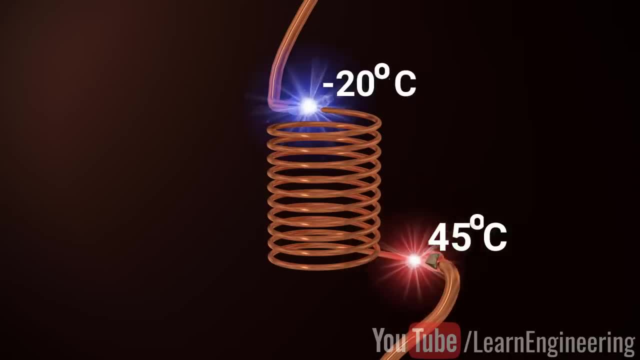 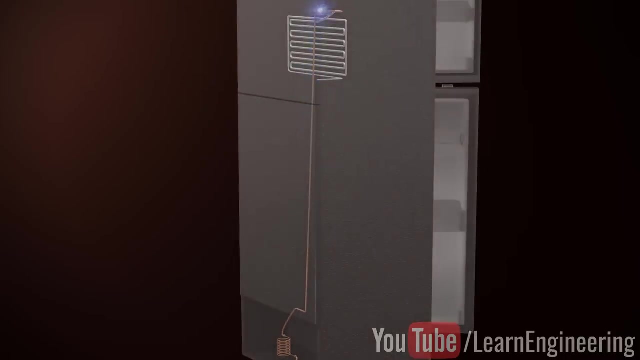 you will notice this drop. Please note that only a portion of the refrigerant is evaporated here. This is one important problem when we44 How to use a refrigerant. Thanks for watching. Yeah, we have another cold liquid today. that is going to high the. 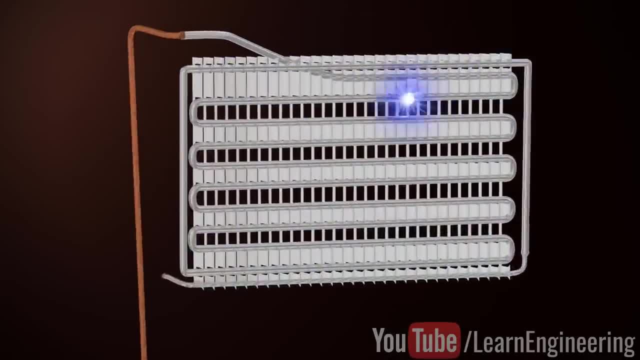 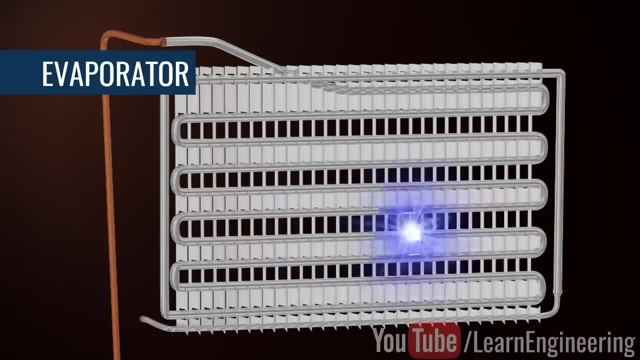 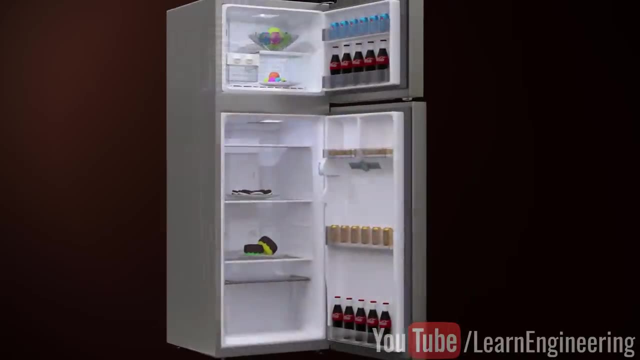 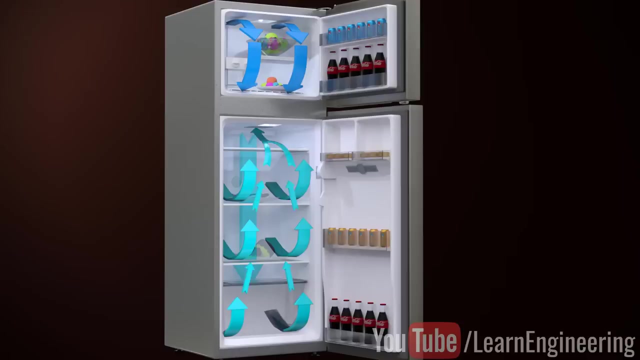 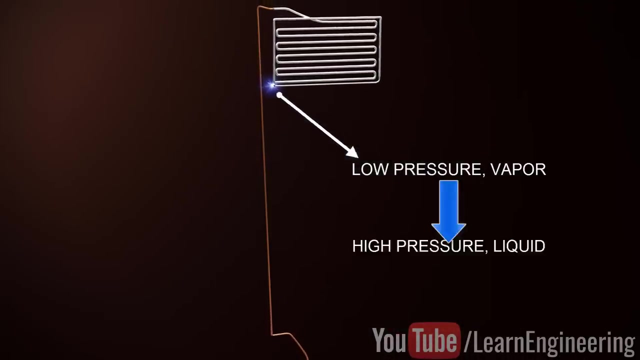 temperature. Siri, can you record something rr is called the evaporator. With the help of clever airflow circulation inside the refrigerator, using an evaporator fan, one can maintain different temperature levels. So we have produced the required refrigeration effect. If we can take this low pressure refrigerant to the state before throttling, that is high. 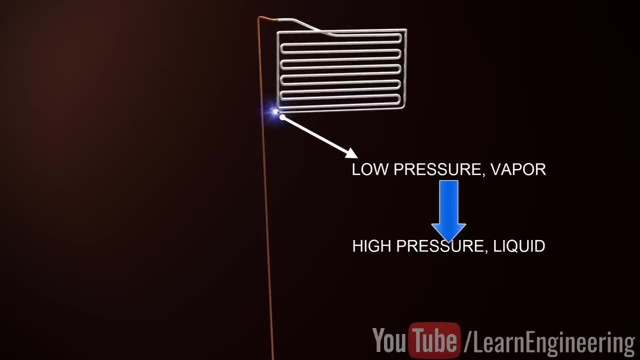 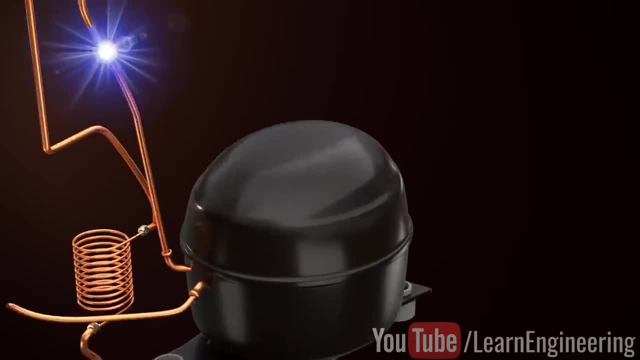 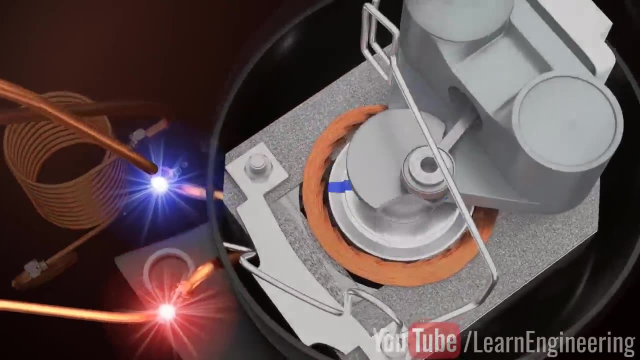 pressure liquid. we will be able to repeat this process. So the first step is to raise the pressure. A compressor is used for this purpose. The compressor will raise the pressure back to its initial value. You can see that a reciprocating type compressor is used here. 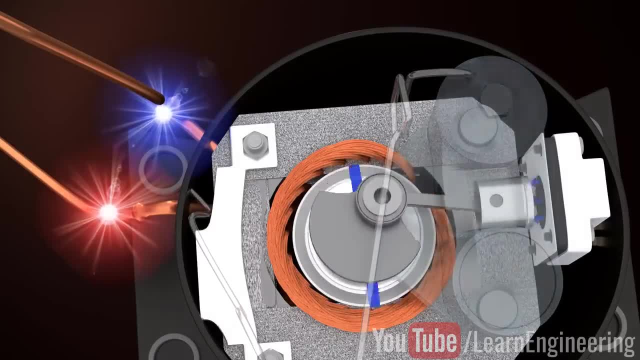 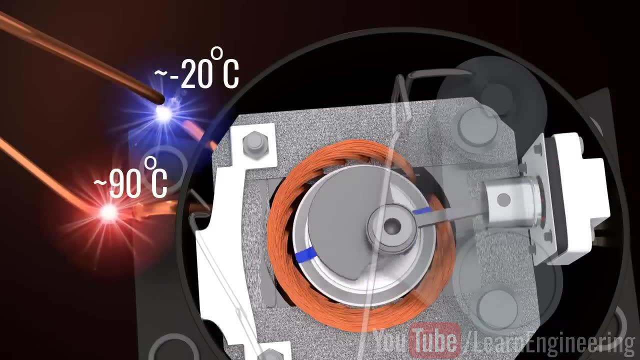 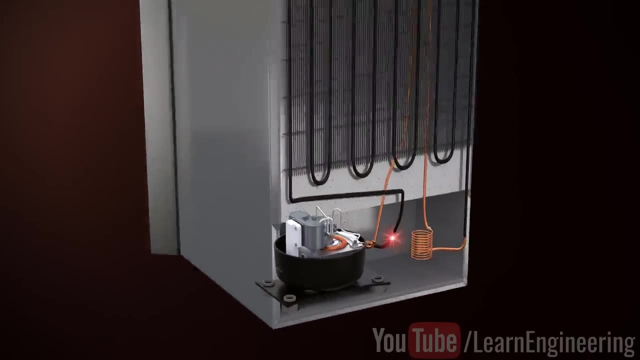 However, since it is compressing gas along with pressure, the temperature will also increase. This is unavoidable. Now the refrigerant is high pressure vapor, To convert it to a liquid stage, we introduce another heat exchanger. This heat exchanger is fitted outside of the refrigerator. 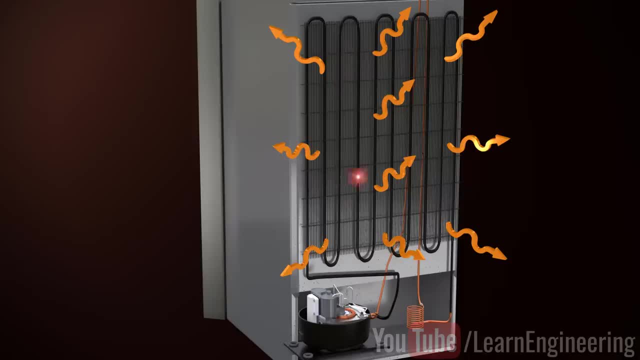 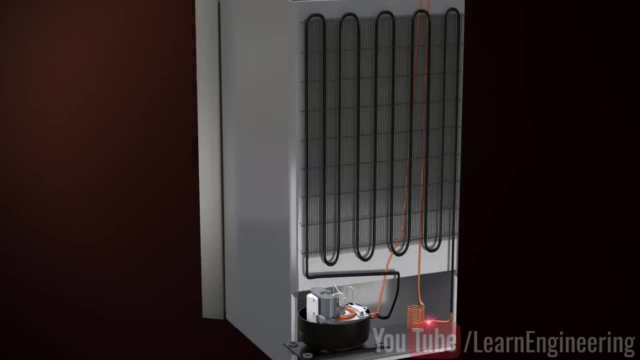 Thus it will liberate heat to its surroundings, Vapor will be converted to liquid and temperature will reach a normal level. This heat exchanger is known as a condenser. Now the refrigerant is back to its initial state, so it can be fed to the throttling. 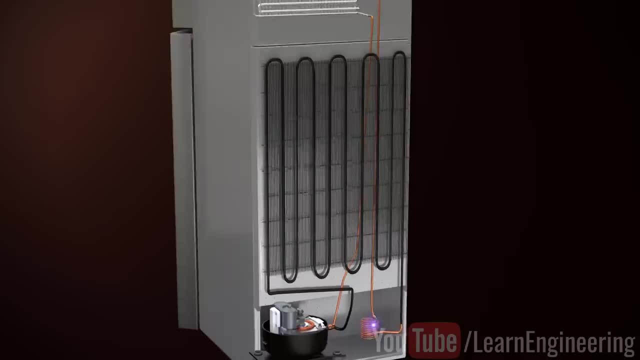 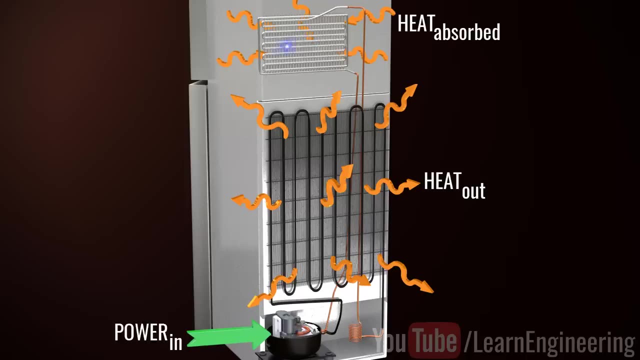 device again. Just by repeating this cycle over and over, we will be able to achieve a continuous cooling effect. This cycle is more specifically called the vapor compression cycle. Refrigerator performance can be evaluated. It is evaluated using a term called coefficient of performance. 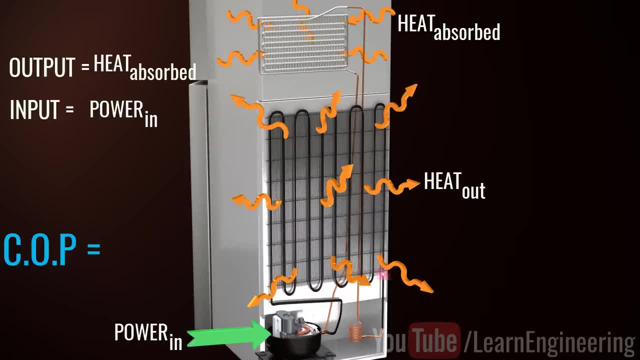 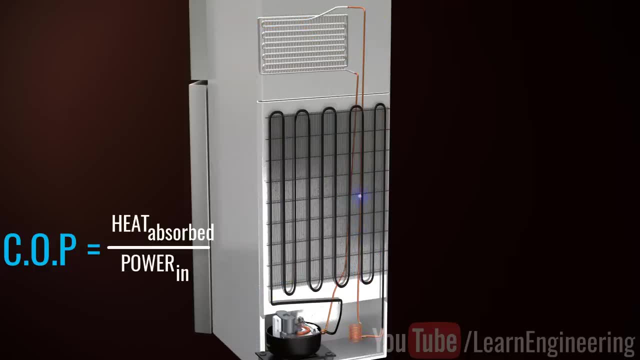 Performance is output divided by input, so the coefficient of performance can be easily defined as follows: This is the most basic refrigerator possible ever. This refrigerator will work well in theory. however, in practice it will face many issues. Let's see what these issues are and how to overcome them. 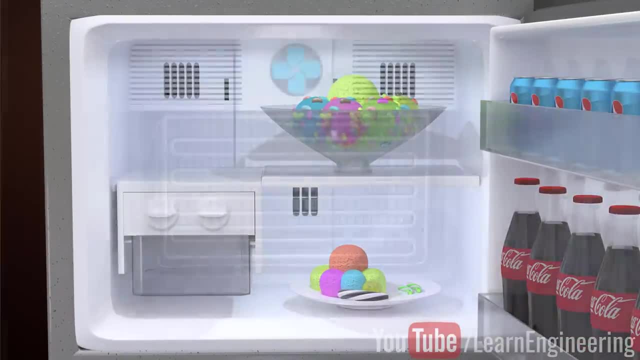 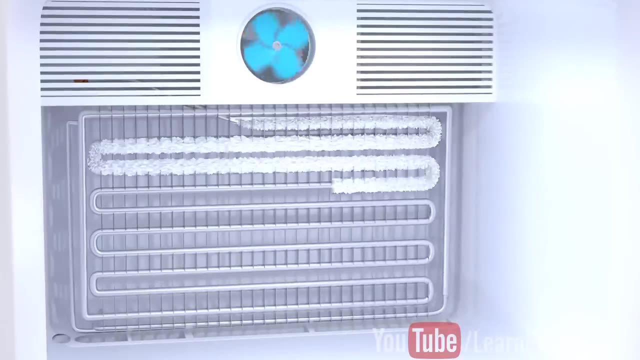 One major issue is the frost developed in the freezer compartment. This is a very common issue in refrigerators. The circulated air has moisture content inside it, So when the air comes in contact with the cold evaporator coil, they will condense and form a frost around the coil. 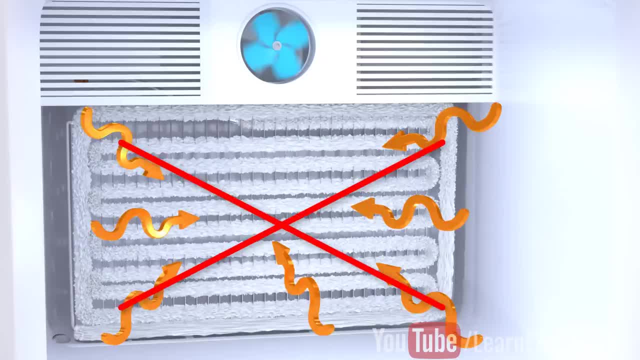 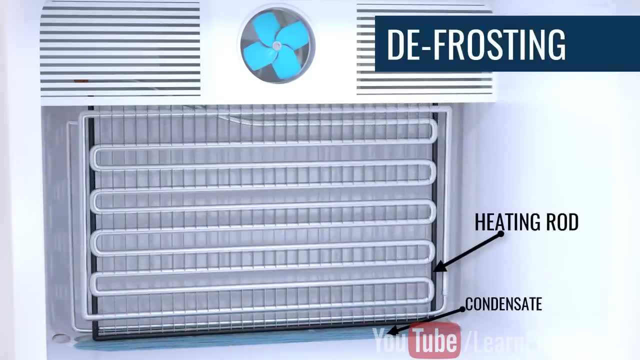 Such ice coating prevents further heat transfer and the refrigerator becomes inefficient over time. One great way to solve this issue is to remove frost, occasionally with the help of a heating rod. This is why you can see a pan and water condensate at the bottom of your refrigerator. 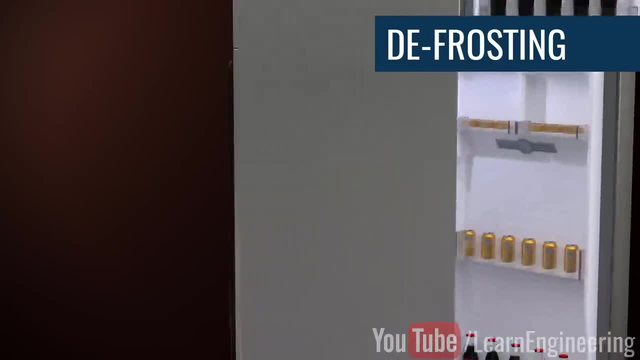 This is the reason you can see a pan and water condensate at the bottom of your refrigerator. The refrigerators are also very resistant to frost. The air is also very resistant to cold and it is also very sensitive to cold. This is a major issue in refrigerators. 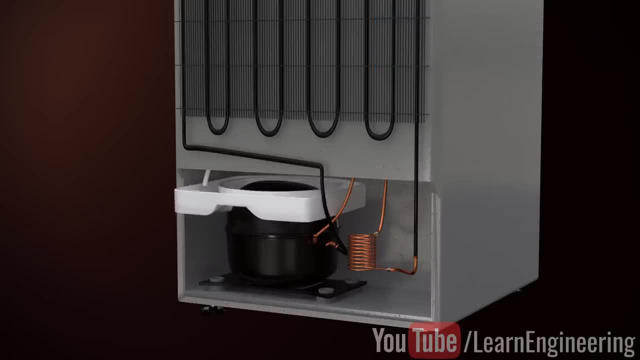 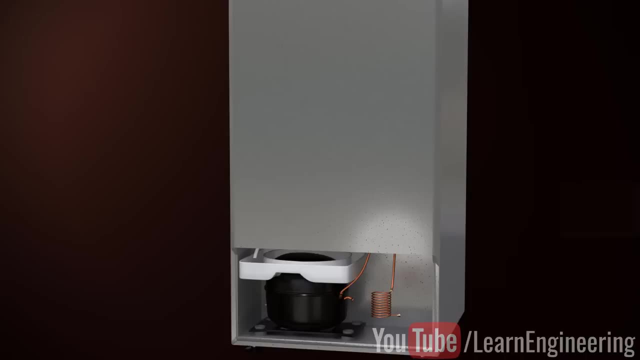 Moreover, in modern refrigerators, you won't be able to see the condenser fins at the back of the refrigerator. Instead, they use a compact condenser arrangement. This compact arrangement is assisted by a cooling fan and the same heat rejection purpose. 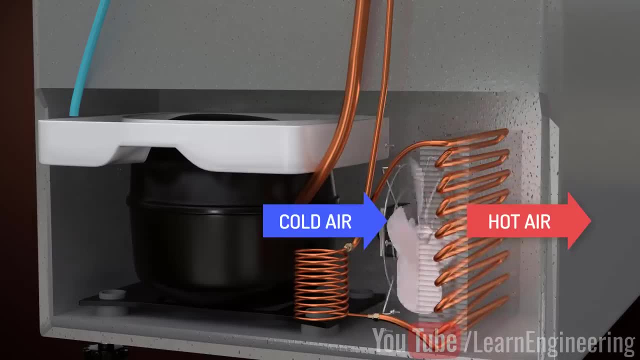 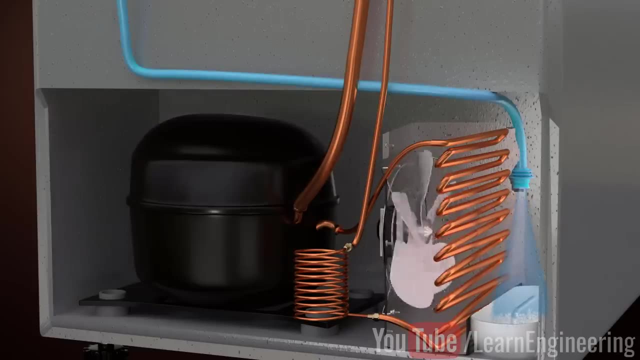 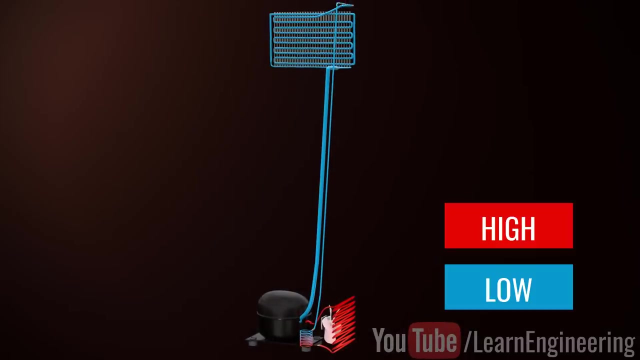 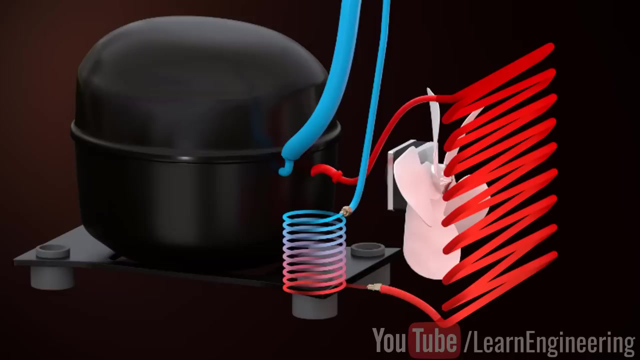 is achieved here. The hot air expelled by the fan can be used to effectively evaporate the water condensate formed during defrosting. The improved refrigerator looks like this. An interesting temperature distribution in different parts of the refrigerator is illustrated here. The temperature drop across the capillary tube is also clearly depicted here. 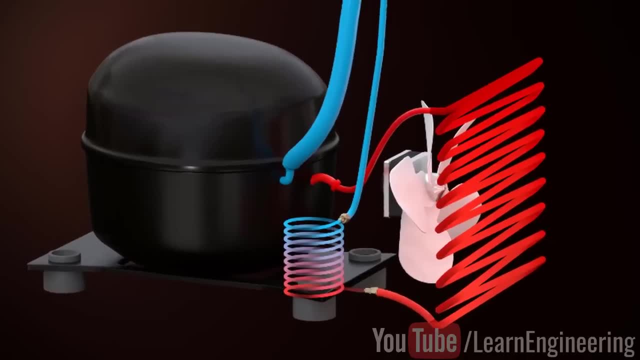 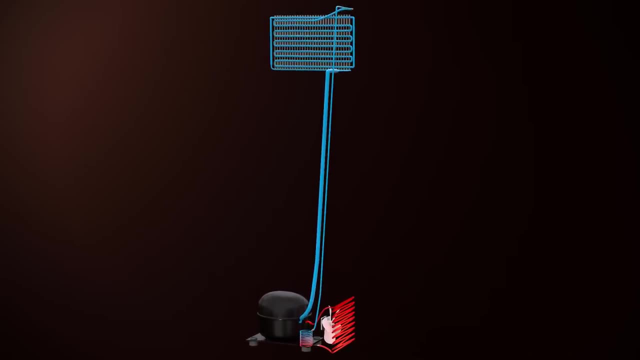 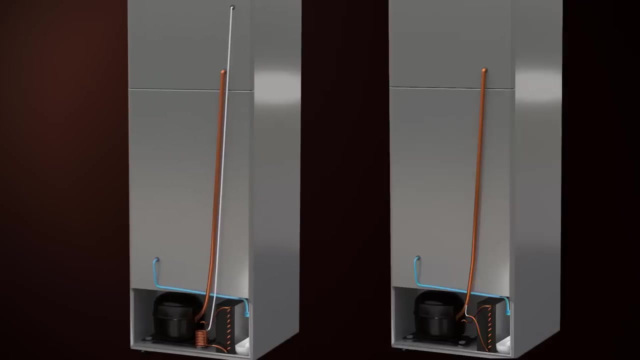 You can see two refrigerant lines outside the refrigerators. One takes the cold liquid from the capillary tube to the evaporator coil and the other the exit vapor line from the evaporator. However, if you check your home refrigerator, you can see only one line on the outside. 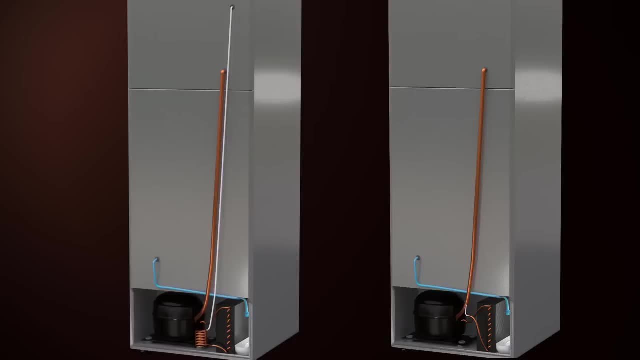 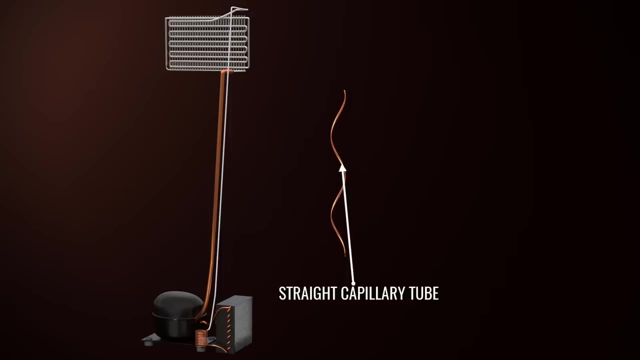 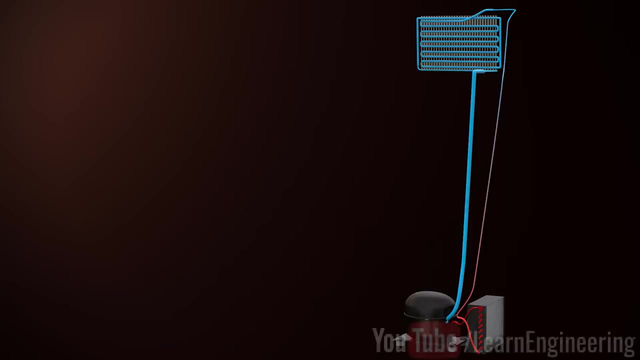 Why is this the case? The most crucial part of the refrigerator is the capillary tube, which need not be a spring-like device. It can be a long straight tube, as shown. Temperature variation in the new straight capillary tube is depicted here. 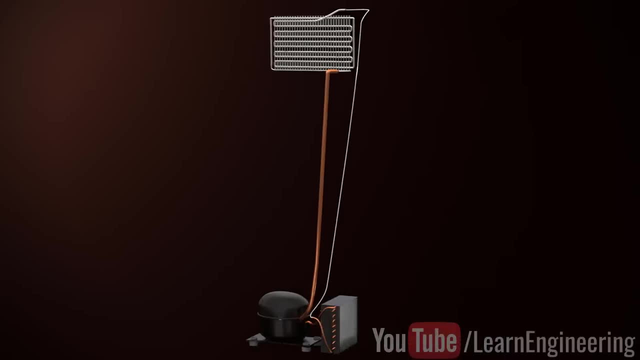 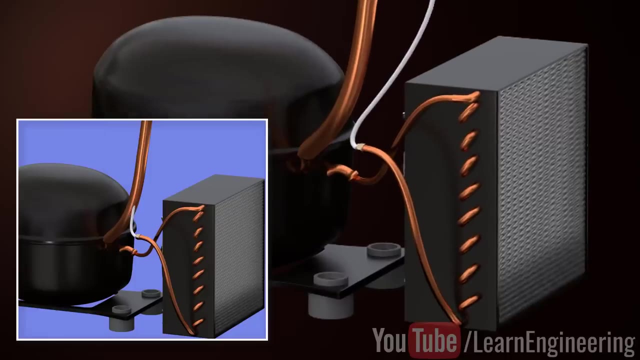 You see only one line on your home refrigerator. This is because the capillary tube is not a spring-like device. This is because this straight capillary tube runs inside the evaporator exit coil. This simple technique has major advantages. We know that during the heat absorption process at evaporator, the refrigerant temperature 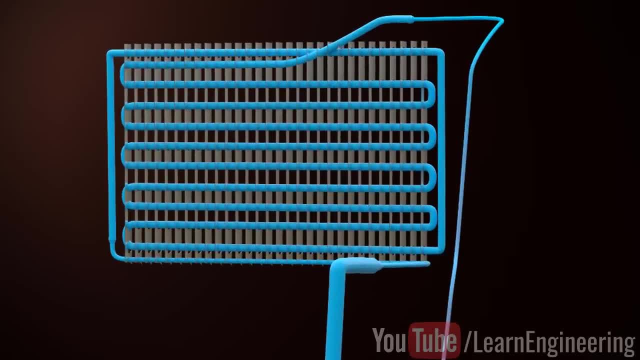 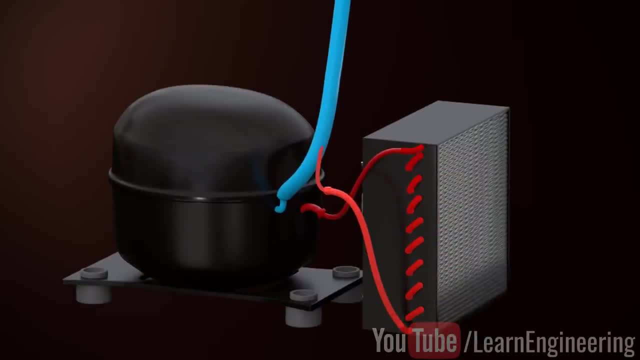 does not rise, only its phase changes. This means that if we allow the capillary tube to come into contact with the evaporator exit line, this will bring down the capillary tube refrigerant temperature by a great degree. This, in effect, will lead to greater temperature drops in the capillary tube, thus creating 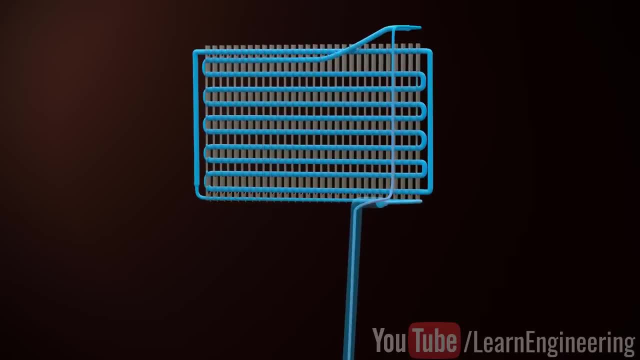 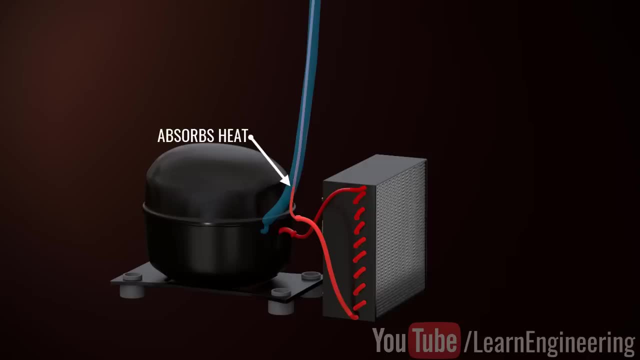 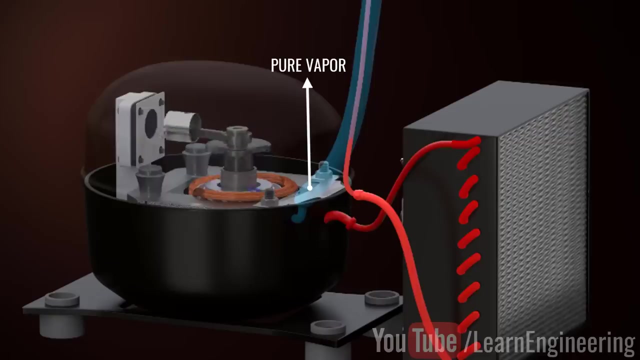 a better refrigeration effect. On the other hand, the evaporator exit coil absorbs heat. This will ensure that the refrigerant in the evaporator exit line has transformed into pure vapor. This is good for compressors, which are designed to handle only pure vapor. 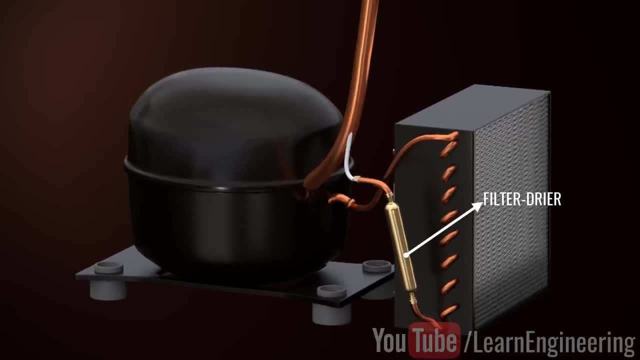 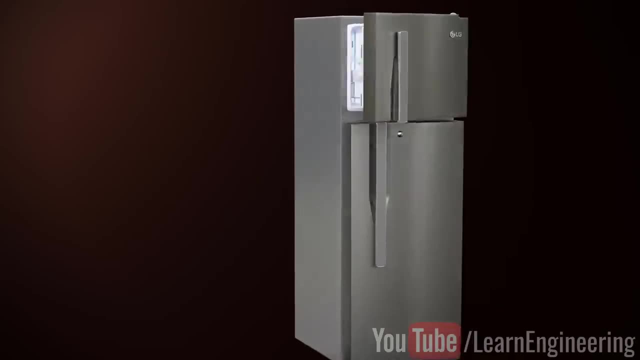 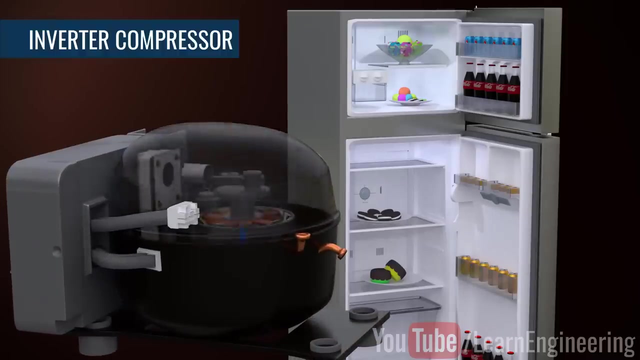 A filter dryer is used to remove any moisture contents in the refrigerant which might become trapped in the compressor operation. Let us now explore the most recent innovation in refrigerators, which has transformed modern refrigerators: Digital inverter compressors. A compressor is the heart of any refrigerator and is the device that gives life to the whole. 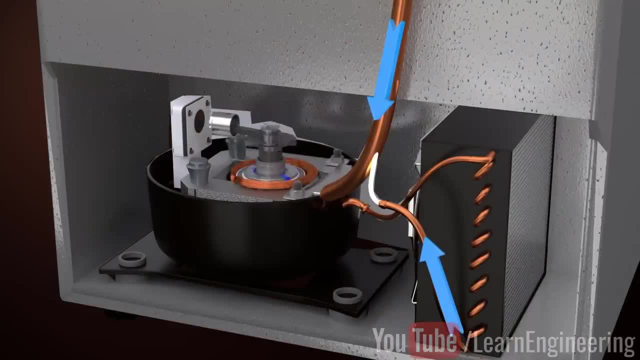 system. You might have noticed that the compressors in old refrigerators will either be on or off. This is a single-speed technology. When the inside temperature of the refrigerator reaches an optimum level, the compressor will be turned off. When the temperature goes above a certain temperature, the compressor will be turned. off. When the temperature goes below a certain limit, the compressors will be turned on. So you can see that the temperature control inside the refrigerator is not smooth. Moreover, such abrupt speed variation of the compressors will lead to durability issue to the compressor components. 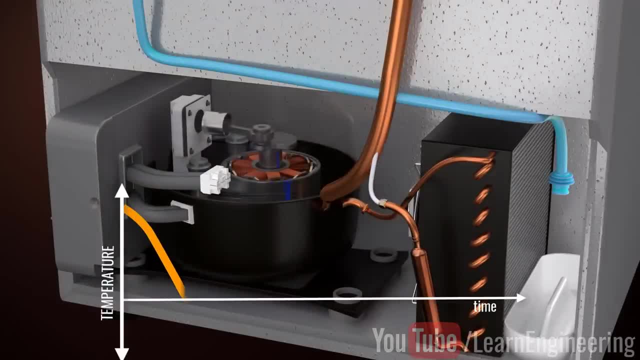 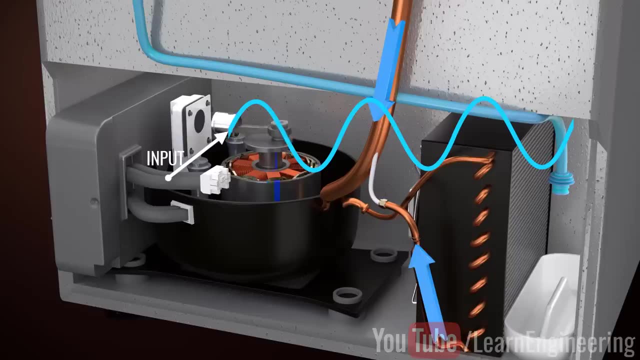 With the help of digital inverter compressor, a variable compressor speed is possible. Thus a smooth and efficient evaporator temperature control can be achieved here. Here the AC power is converted to DC using a controller. The controller then supplies electric power in variable frequency to accurately control.